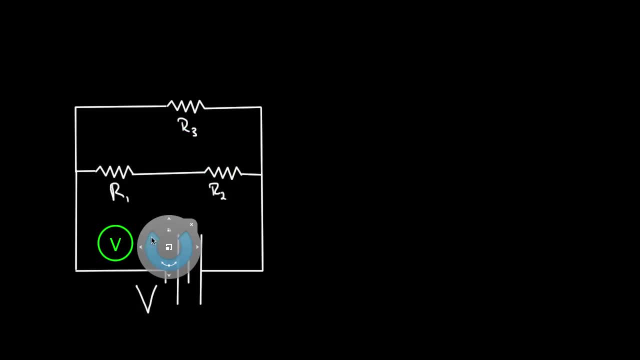 Or take the voltmeter, put it over here and if I connect the leads across R1 in parallel, notice I'm hooking up the voltmeter in parallel. Voltmeters you always hook up in parallel. This now will tell me the voltage across R1,. 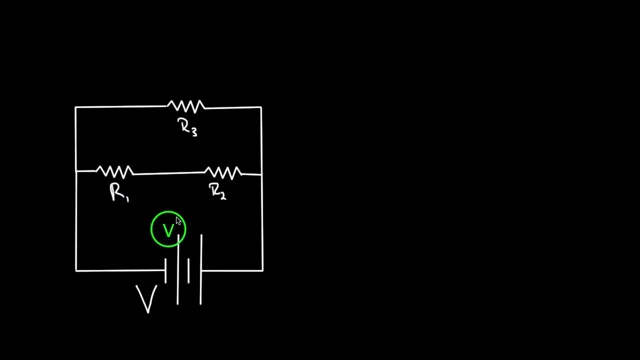 and if I wanted to make sure my battery was functioning correctly, I could take my voltmeter and I can hook up the leads across the positive and negative terminals of the battery and see if the voltage across the battery is what I think it is. 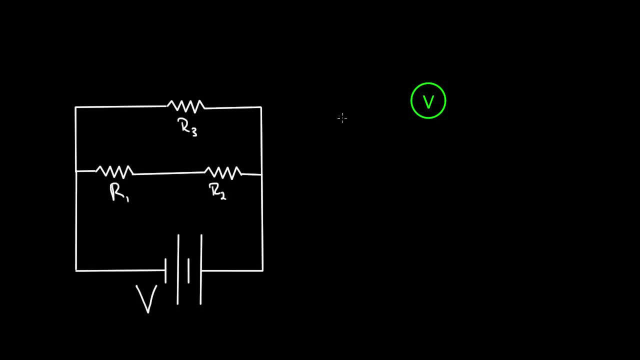 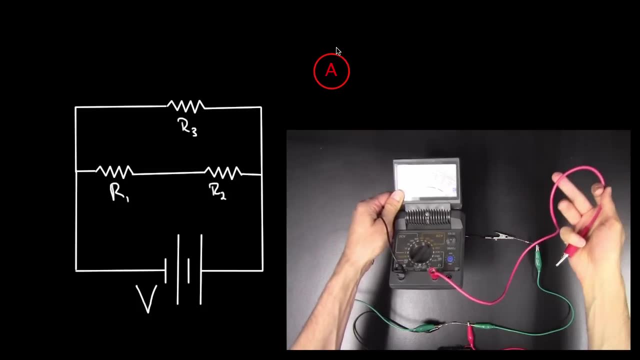 That's how you use a voltmeter, always hooked up in parallel. But if I wanted to measure the current, I don't use a voltmeter, I use an ammeter, And for an ammeter you do not hook up an ammeter. 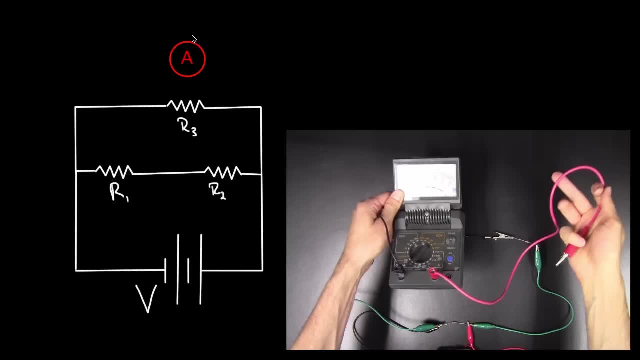 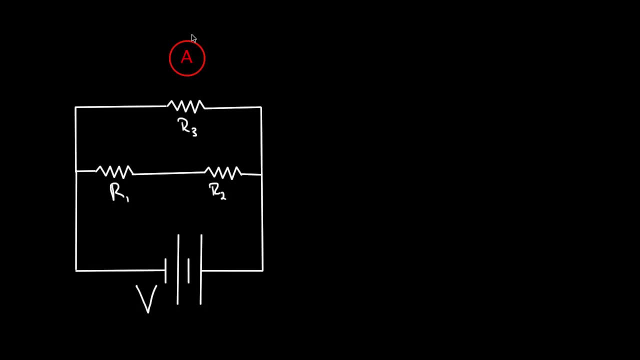 in parallel with the element you're trying to measure. in parallel, You'll probably blow out the ammeter. I've done it a few times. it's embarrassing. Don't hook up the ammeter in parallel. I'll tell you why in a minute. 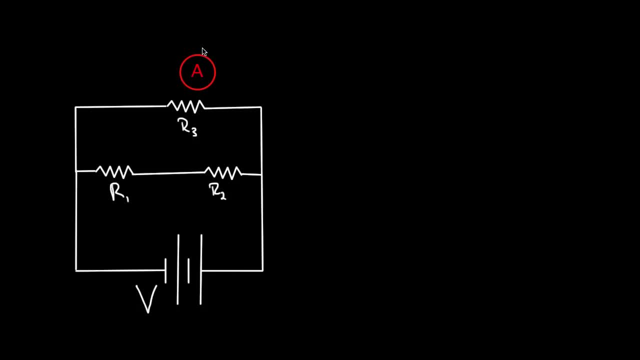 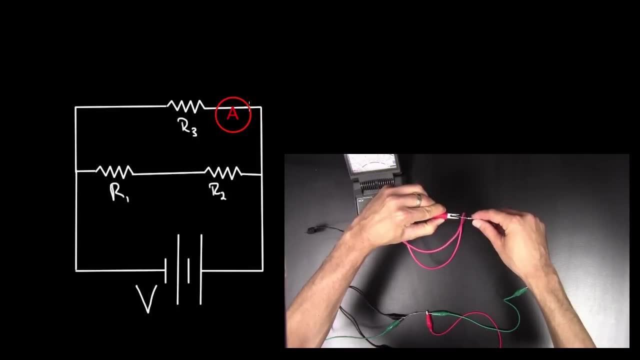 But what you have to do is hook it up in series. So if I wanted to know the current going through R3, I could just stick this ammeter right in here. One lead would plug into one side of the ammeter, The other lead would plug into the other side. 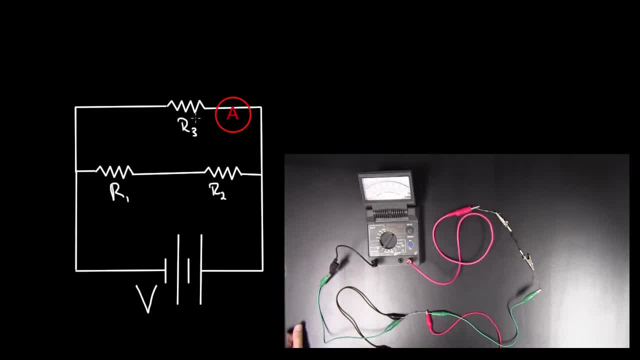 This current would have to flow straight through the ammeter, and this is telling me how much current goes through R3.. It doesn't matter which side I put it on: The current going into R3 will equal the current going out, So I can put it over here too. 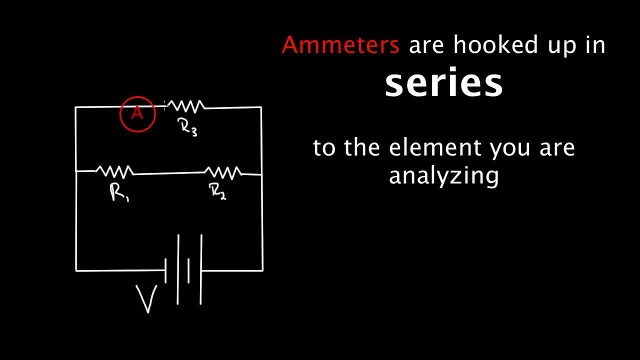 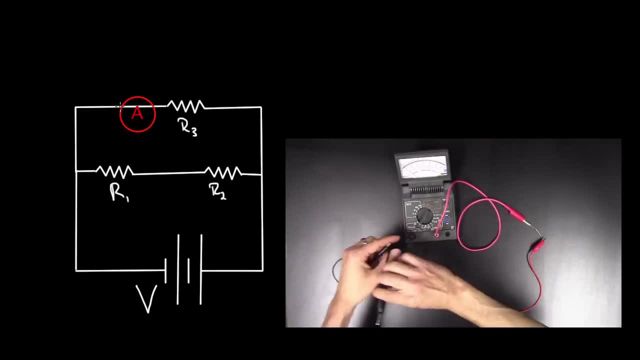 But it's got to be hooked up in series So you have to disconnect. It's kind of a pain to hook up an ammeter. sometimes You have to disconnect something here then connect that connection to the one side of the ammeter. 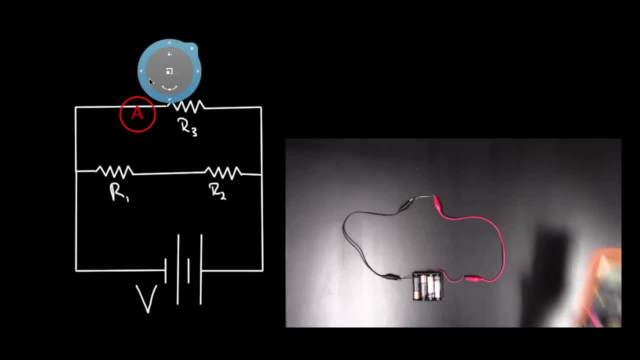 connect to the other side of the ammeter For a voltmeter. you didn't have to do that For a voltmeter- voltmeter, you just kept it out here and just touch those leads wherever you needed to touch them. 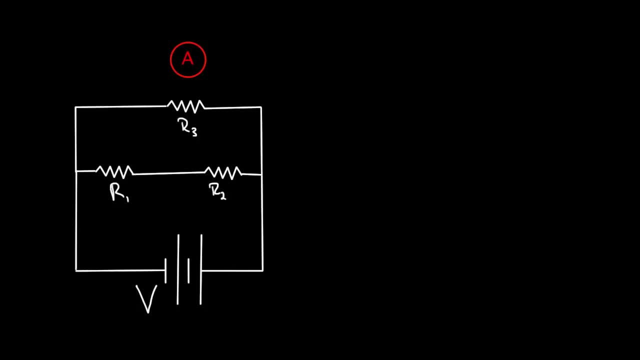 But for an ammeter you have to break the circuit to let this ammeter in. But I can move it wherever I want. I can put it down here. That tells me the current in this strip. Again, ammeter's always hooked up in series. 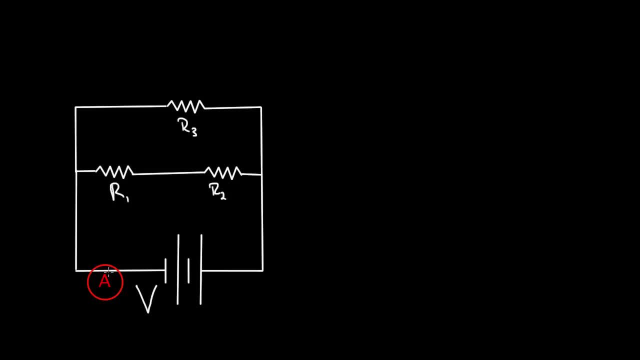 with the element that you're trying to measure. So this ammeter position will let me measure the current that's flowing through the battery. But why is the voltmeter always hooked up in parallel and the ammeter always hooked up in series? We want the ammeter to be hooked up in series. 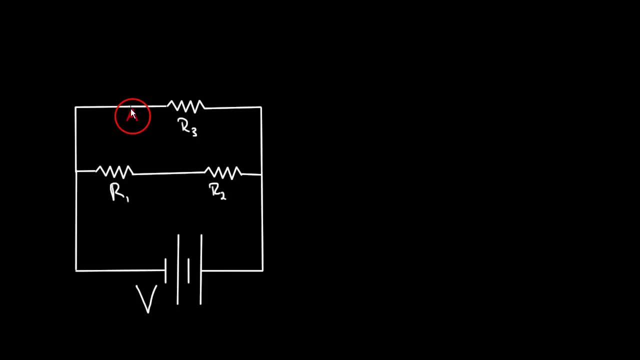 because we want to measure the current through a line in the circuit. We want to measure the current flowing through this resistor. So if we want to measure the current flowing through something, we need to make sure that the current flows through our ammeter, and that's how we get our reading. 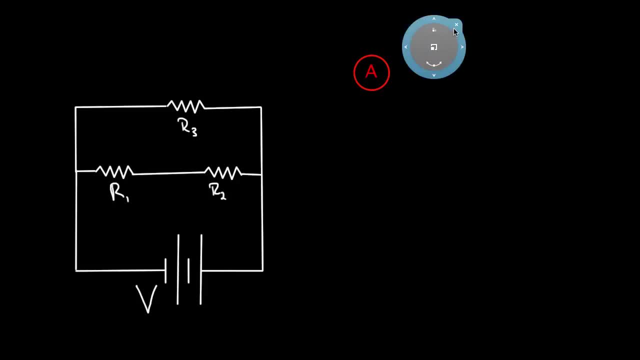 Because of this, people design ammeters with very little resistance. An ammeter has very little resistance And the reason is, if you took this ammeter and it had a big resistance and you stuck it in here, you'd be changing how much current flowed. 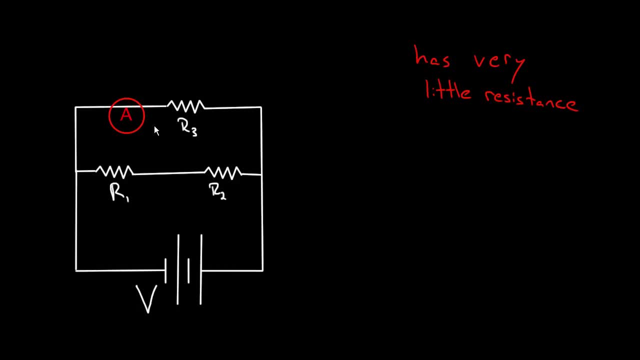 through this part of the circuit. We don't want to do that. Whenever we measure something, we don't want to disturb it. So when I stick my ammeter in here, I don't want to disturb how much current was going through here. 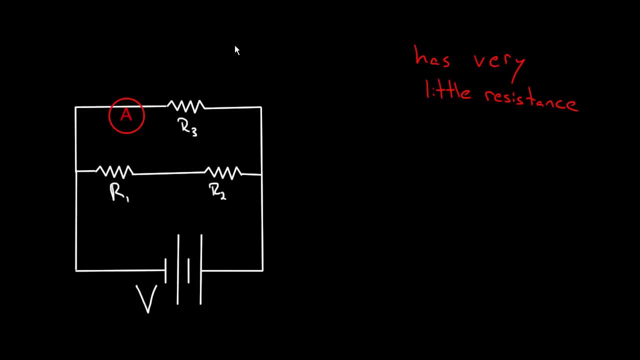 I wanted to know how much current flows without my ammeter being in there. When I put my ammeter in there, it better have very little effect on this circuit. That's why we make this ammeter have a very small resistance And that's also why you can't hook this ammeter up. 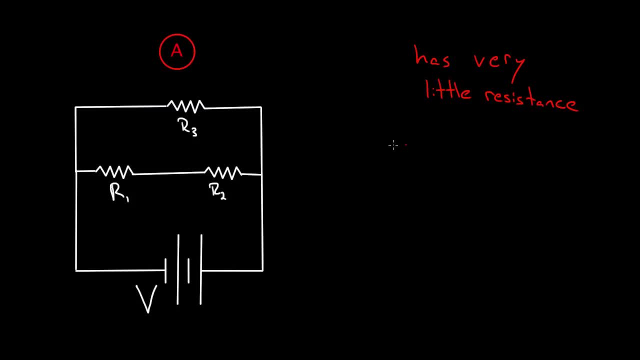 in parallel, because if you did, look at what would happen. This is why it's bad If I took this ammeter and I hooked it up right here and I hooked it the other side up right here. look what the current's going to do. 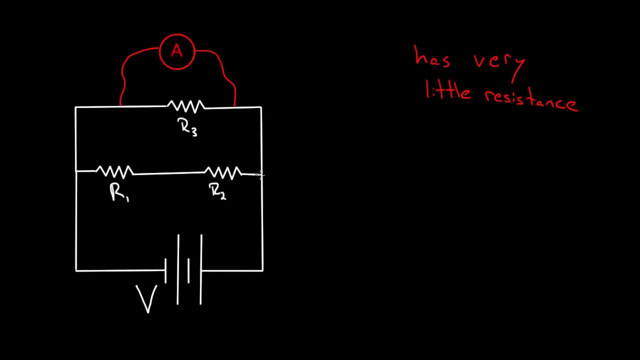 I've got current flowing through here. Current comes this way, goes this way, reaches this fork in the road and it's got a choice: It can go to the left or flow up through here and go through R3. Or flow through my ammeter. 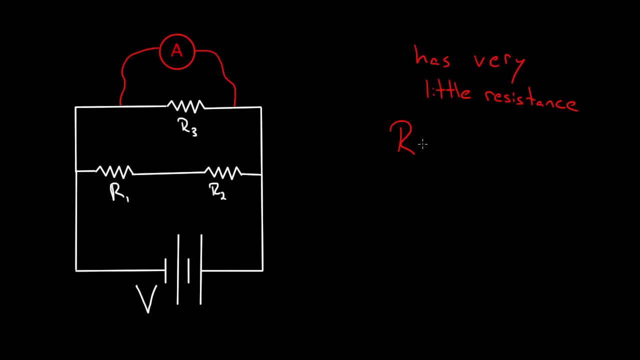 But my ammeter has very little resistance. I mean small, maybe on the order of a milli-ohm. So all of this current that's flowing through here, all this current's going to choose to go through my ammeter. It's going to just skip all those resistors. 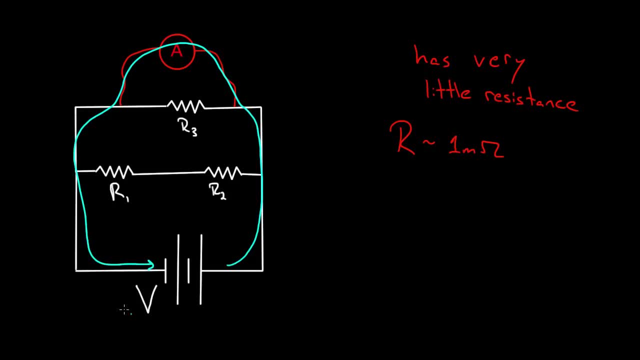 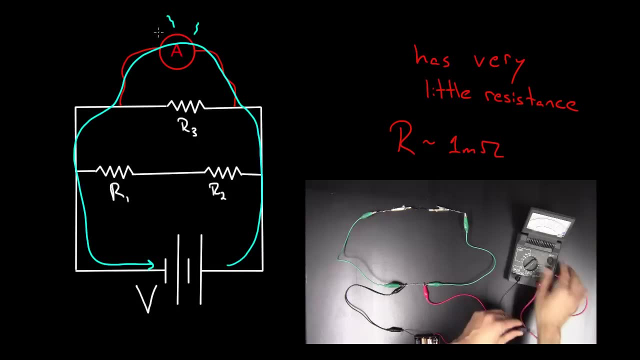 Forget that. It just goes through the ammeter. If you've got a normal sized voltage, maybe nine volts, three volts hooked up to a milli-ohm, you're going to burn out your ammeter. There's usually a fuse in here, because they know. 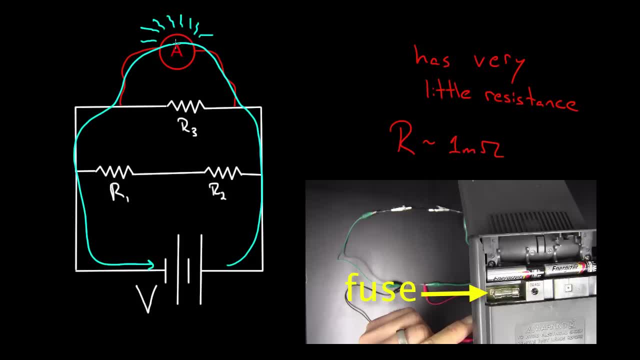 people are going to hook it up wrong. I've done that And you burn out a fuse. you've got to go replace the fuse and it's a pain. So don't hook up your ammeter in parallel. What about voltmeters? 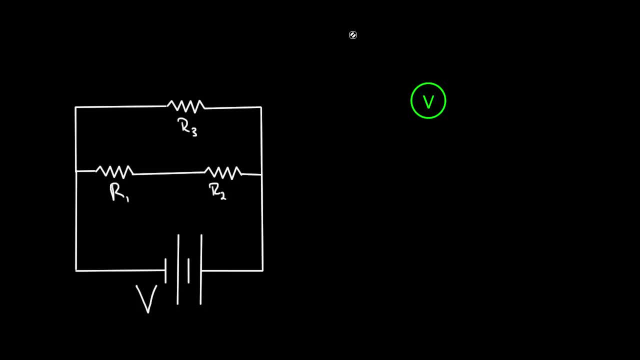 Why do we hook those up in parallel? Well, a voltmeter's hooked up in parallel because we want to know the voltage across a circuit element. So on either side, Voltage, remember, is defined to be the difference between electric potential at two points in space. 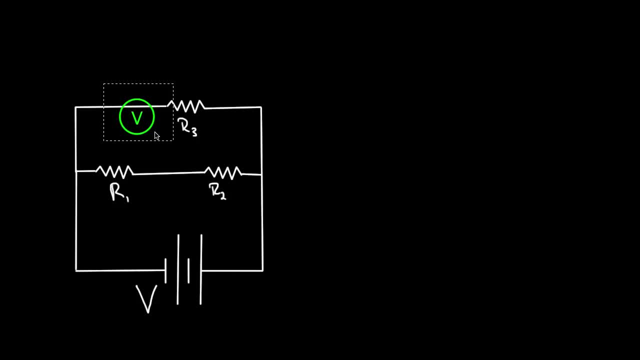 It makes no sense to ask what's the voltage through a certain point in a circuit. You can ask what current flows through that point in the circuit, But asking what the voltage is at a particular point in a circuit makes no sense. The only thing that would make sense is asking: 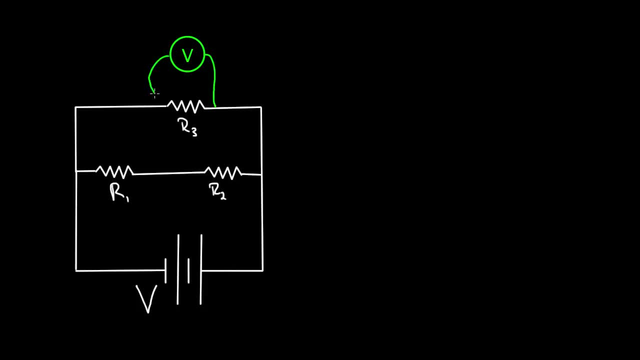 what's the voltage across two points in a circuit. So I can ask what's the voltage between this point and that point? That makes sense. Or I can ask what's the voltage between this point and that point? That makes sense. 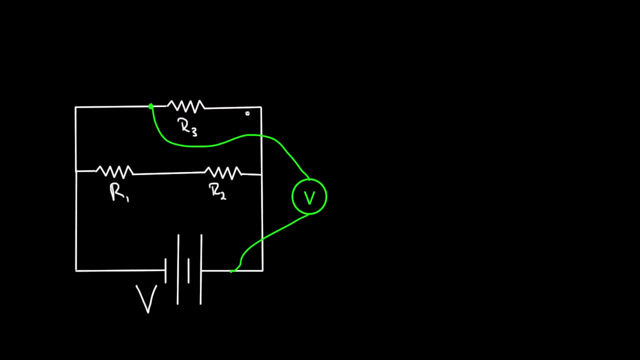 But asking what's the voltage at a point or through a point makes no sense. That's what current is. Current flows through a point. Voltage is across another point, across two points: the difference in electric potential between two points. That's why we hook up volt meters in parallel. 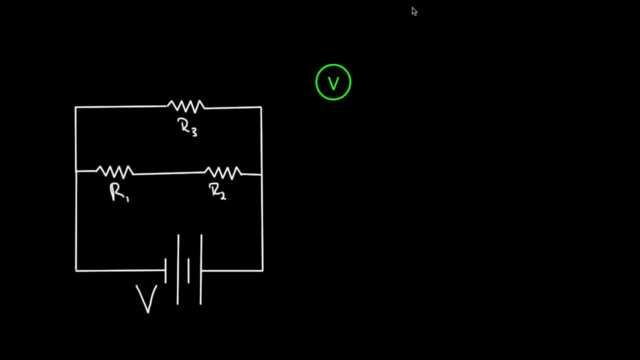 And because we hook up volt meters in parallel, volt meters have to have a huge resistance, sometimes on the order of hundreds of thousands of ohms or even millions of ohms. So this can be big, big number of ohms. And the reason is: think about it. 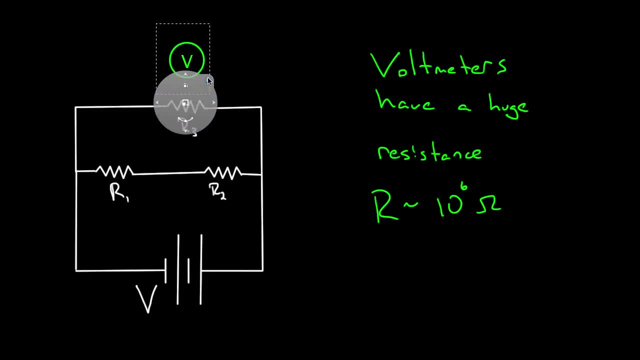 again, our key idea is that we don't wanna disturb the thing we're measuring. I'm measuring the voltage across this resistor. If I were to hook up a volt meter with very little resistance, I just told you what would happen: This current that's flowing out of the battery. 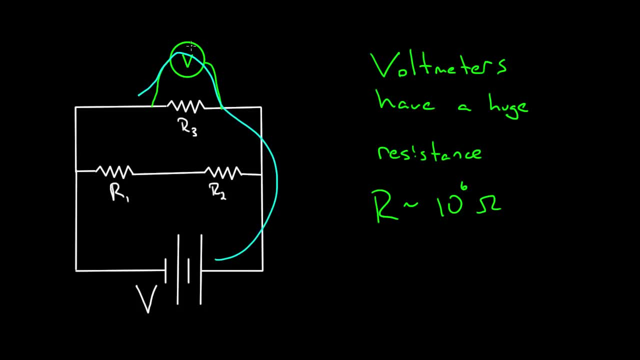 would all try to go through this volt meter. It would. not only would it try to mess up the volt meter, but that's current, that's not flowing through R3 anymore, and so I wouldn't get a correct reading for the voltage through R3.. 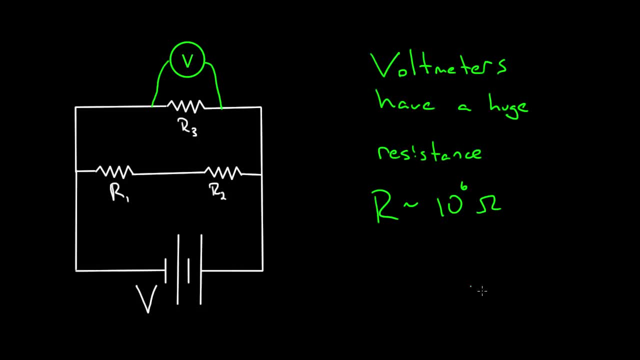 So we wanna make sure our volt meter has a big resistance so that, yes, I mean technically a very, very small amount of current- maybe a milliamp- will flow through this volt meter because it's gotta take a reading. but we want a small amount of current. 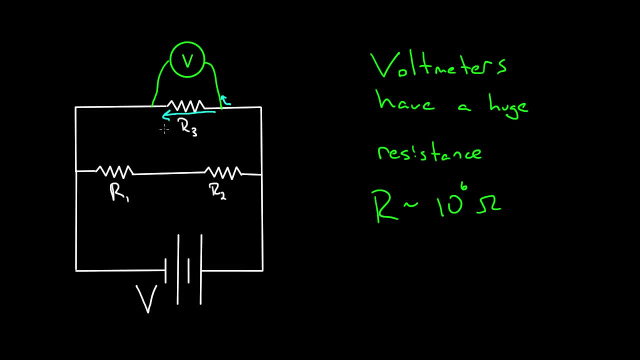 as round as possible, because we wanna keep this current flowing through R3 the same as it was before we were measuring it, because I know V equals IR and if I can measure this voltage across here, I wanna make sure the current's the same or I won't be getting an accurate measurement. 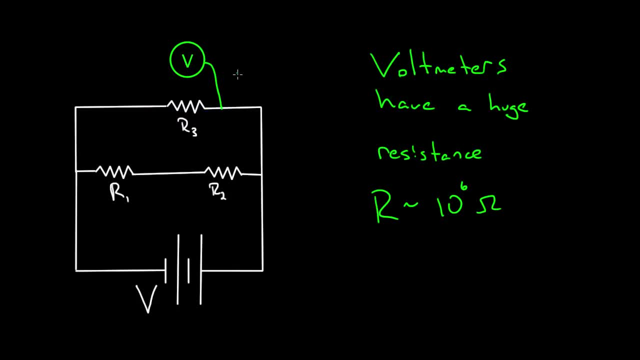 for the voltage. You could ask what would happen if we did hook up the volt meter in series instead of parallel. Volt meters have a huge resistance, so if I stuck that here, the volt meter has a huge resistance, You wouldn't break it.